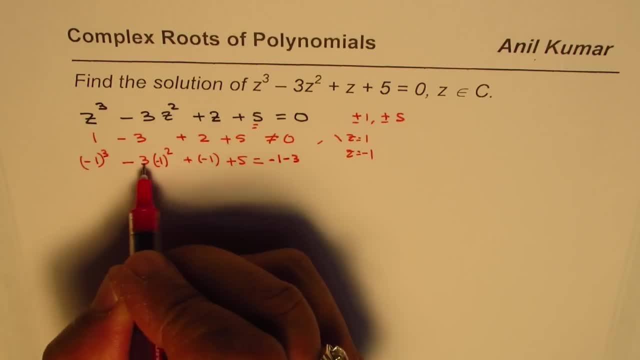 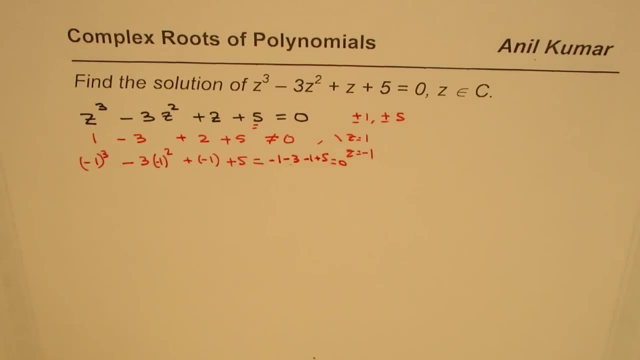 This is minus 3, and that gives us minus 1 plus 5.. So that, indeed, is equal to 0.. So minus 1 works right. So what we find is that the value of this polynomial is 0 for z cube minus 1 square plus minus 1 square. 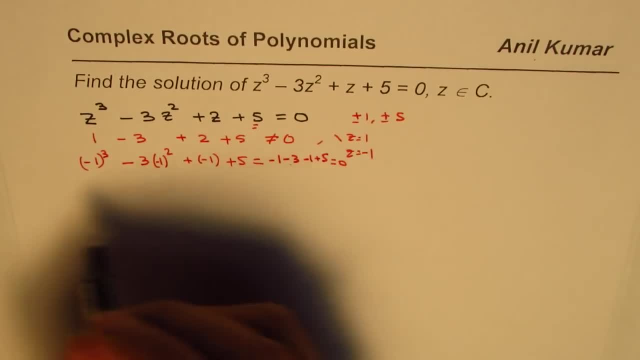 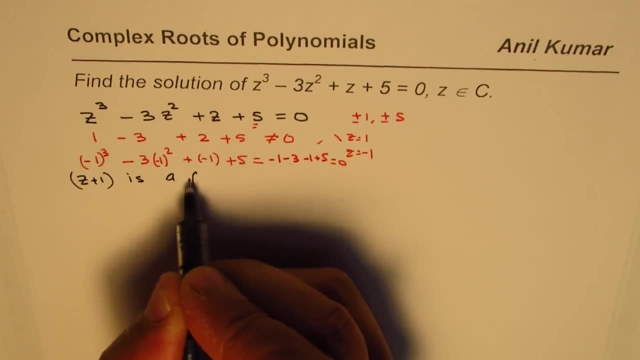 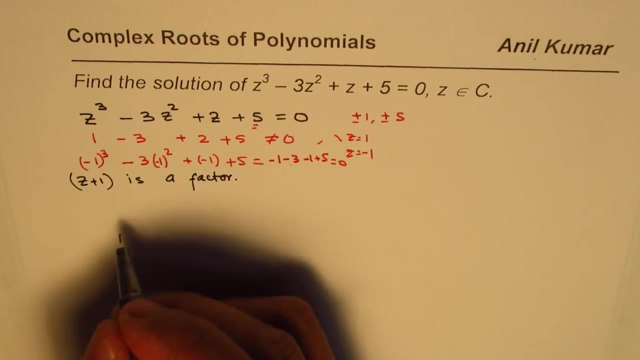 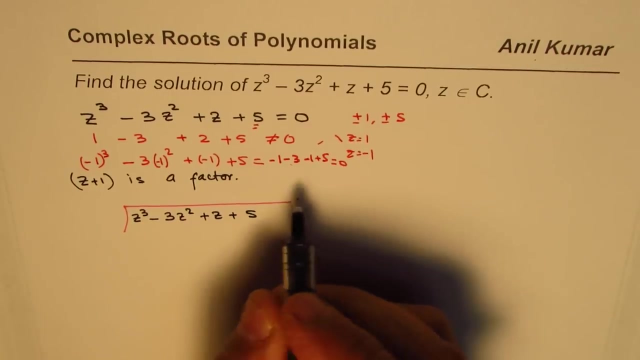 is 0 for z equals to minus 1 and that means that z plus 1 is a factor right is a factor to find the other factors. we can do long division right. so let's do long division to find the other factors. so we'll divide z cube minus three, z square plus c plus five by 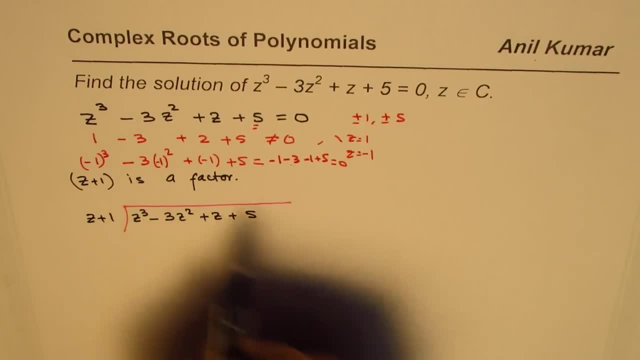 C plus one. so you could do- let me use a different ink- Z square, so that gives us Z cube plus Z square. when you take away, you get minus 4 z square plus z. so we could do now minus 4 z. so that is minus 4 z square, minus 4 z. 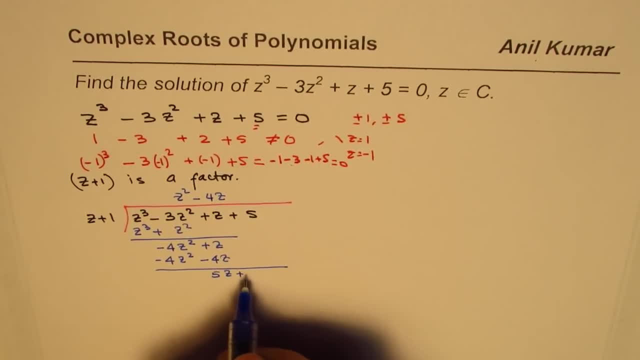 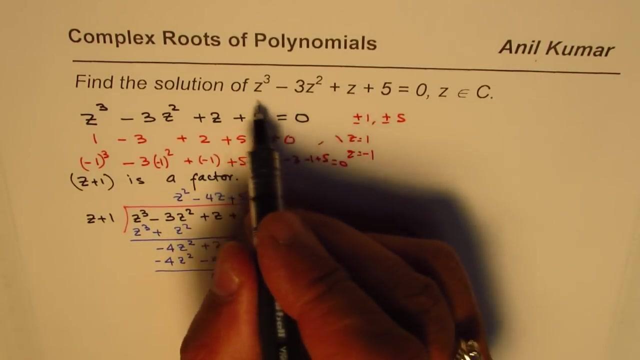 and that gives us 5 z plus 5 plus 5. so which is 5 z plus 5. so the remainder, as expected, is 0. so that means z square minus 4, z plus 5 is a factor, so i could write this polynomial, let me. 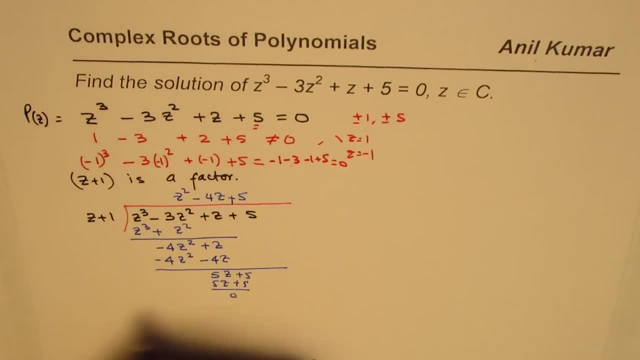 write this polynomial: p of z as equal to p of z, as equals to z plus 1 times the quotient which is z square minus 4, z plus 5. right now, to find the other factors, we could use the quadratic equation and find the factors for z square. let's do that, so we have z square. 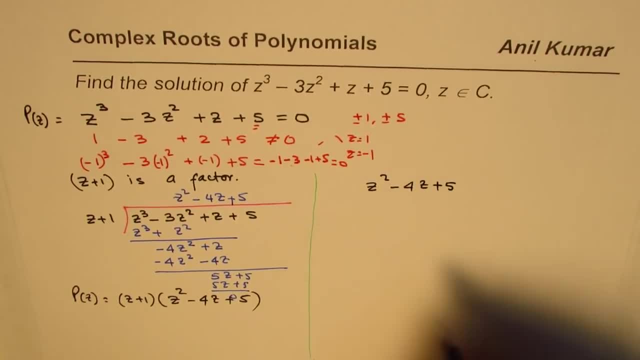 x 4, and then we can find the other зам fusei cube and we can substitute the number between them with the shapes that have e x. we can dramatically subtract a square from that. if you can calculate minus 4z plus 5, we can find the value of z. as you remember the quadratic equation, let me write it.